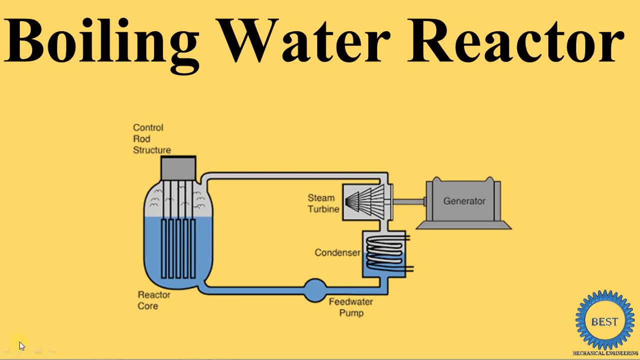 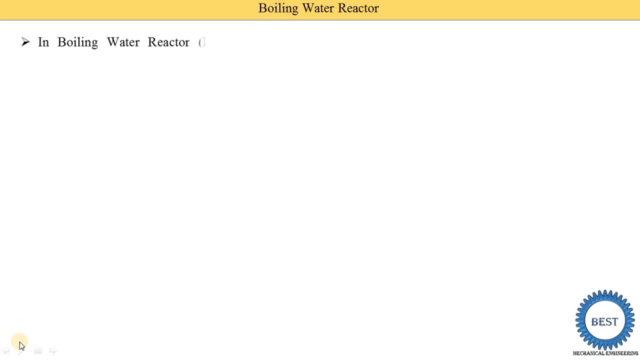 In this video I explain boiling water reactor. it is also known as the BWR. In this video I explain the construction, working, advantages and disadvantages of BWR. So first we understand the constructions of the boiling water reactors. In boiling water reactor, enriched uranium is used. 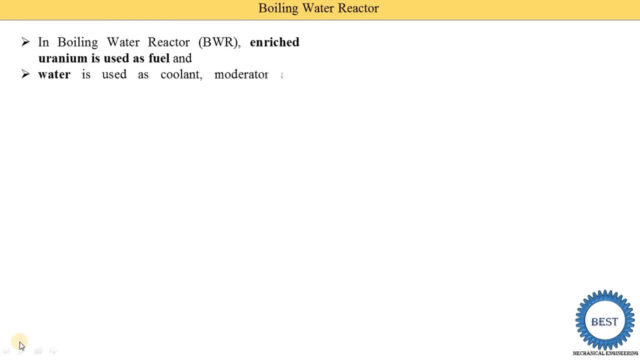 as a fuel and water is used as a coolant, moderators and reflectors, like a PWR. PWR means pressurized water reactor means fuel is enriched, uranium is used as a fuel and water is used as a coolant, moderators and the reflectors, like a PWR Expect. the steam is generated in the reactor. 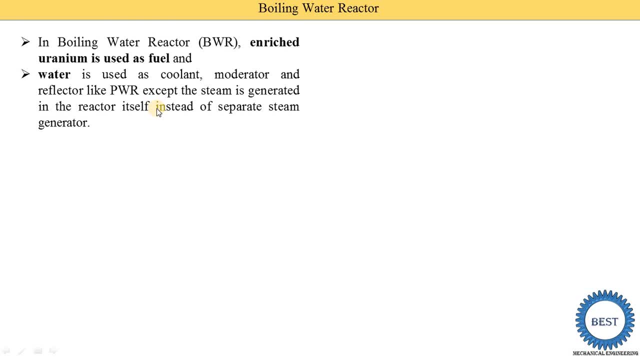 itself, in sense of the separate steam generators. In a PWR the steam is generated in a separate heat exchangers, but in a PWR the steam is generated in the reactor itself, which means the heat exchangers are not required in a boiling water reactors. The arrangement of the boiling water. 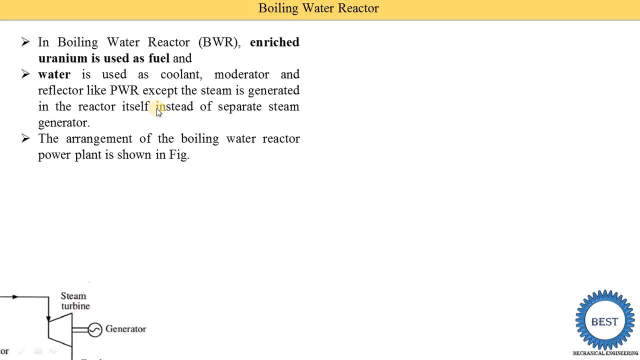 Reactor power plant is shown in these figures. Now, here you see, it is a simple figure of the boiling water reactors. So this is the reactor, This is the reactor. core means the fuel andautres of this reactor. So in theись Data, the power plant resource. 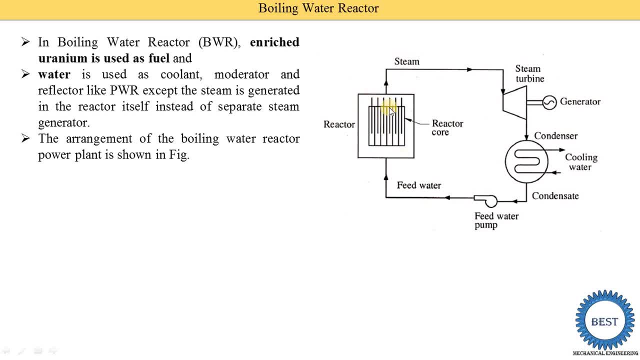 are there and this control road is the reactor course. this water is enter in this reactor and this water is converted into the steam. means the water is absorbed, the heat energy produced due to the fission reactions. okay then, this is a steam turbine condensers and this is a feed water. 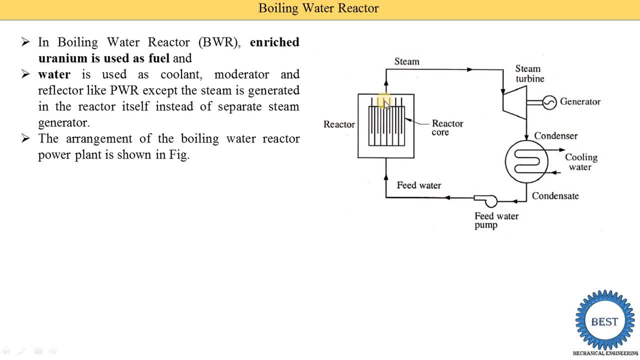 pump. that is only four components are there? okay, means it is a suppose we compare this bwr with the rankine cycles. okay, so in a rankine cycle just we need to replace the boilers by the reactors. okay, then it is. converting to this boiling water reactors means in a constructions you need to. 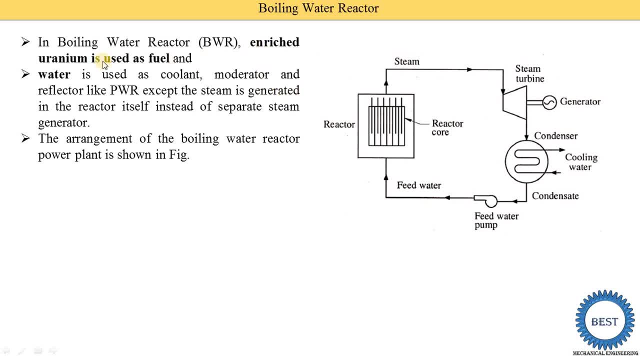 remember which fuel is used that is enriched uranium and water is used as a coolant. modulators and the reflectors and its component are the reactor, steam turbine condensers and the feed water pump. now we understand it's working. the feed water circulated in the reactor. 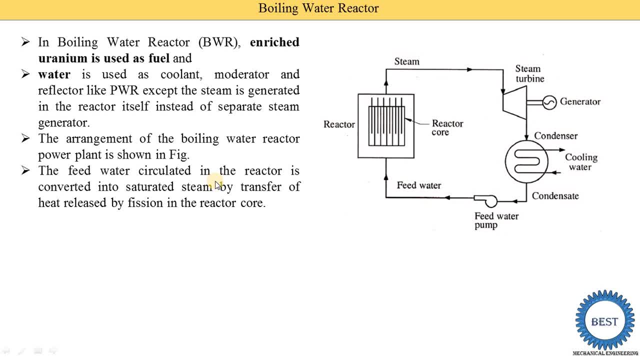 the feed water circulated in the reactor and the feed water pump- now we understand it's working- is converted into saturated steam by transfer of heat release by fission in the reactor codes. so in a reactor code that is, a fuel means the enriched uranium is there. moderator is there. 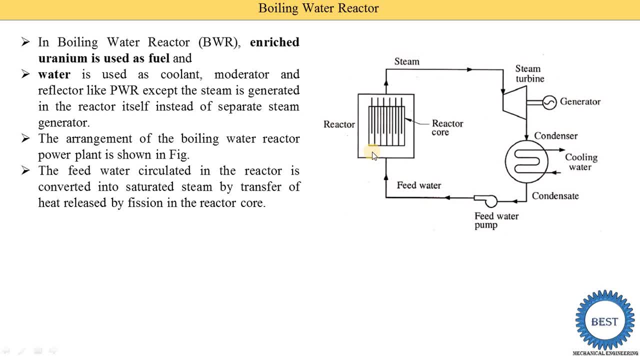 okay, so this fuel is released. the heat energy: okay, and this heat energy is absorbed by this feed water. okay, and this feed water is converted into a saturated steam in the reactor itself. okay, so here you see. outlet from the reactor. is the steam? okay in a pwr, that is, a water is coming. 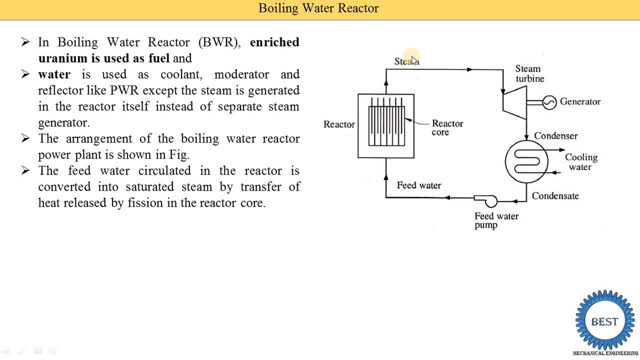 and this water is supplied in a heat exchangers and from the secondary circuits. the water is coming and in a heat exchanger this water is converting, but in the pwr this feed water is directly converted into the saturated steam. this steam is supply to steam turbine working on the 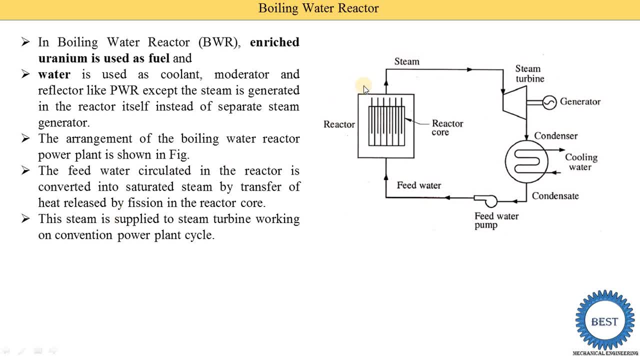 conventional power plant cycles. you means this steam is enter in the steam turbines and the steam is expand and some mechanical work is produced. this mechanical work is supply to the generators and in the generator electricity is produced. and the outlet steam from the steam turbine is supply in a condenser and in a 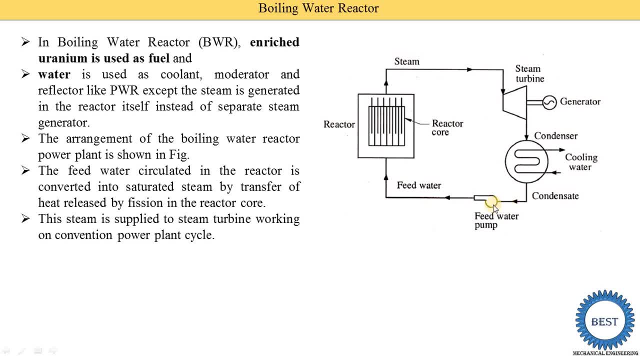 condenser, the steam is convert into the water. this water is supplied in this feed water pump and in a feed water pump, pressure of the water is increased and this feed water is again supplied to this reactor code. this way, the cycle of the boiling water reactor is continuous. the mechanical power produced by the turbine is converted in the 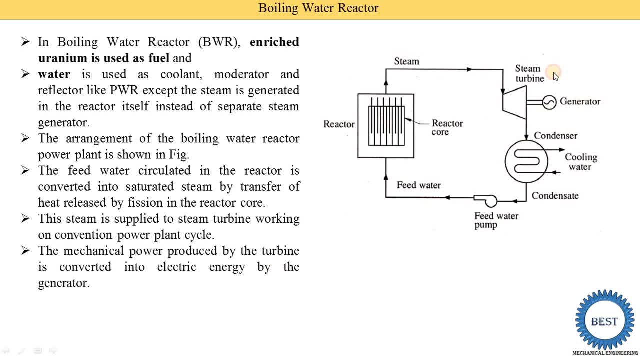 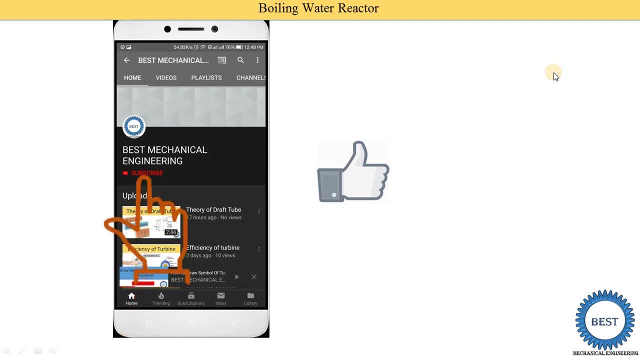 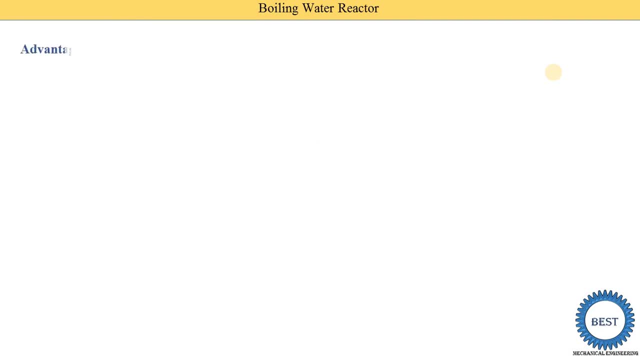 electric energy by this generator. that we already understands. now we understand the advantages and disadvantages before moving ahead. i request to like the video. subscribe my channel for watching the more video related to power plant engineering, another subject of this: mechanical engineering. so first advantage: the pressure inside the reactor vessel is less than the pwr. pwr means 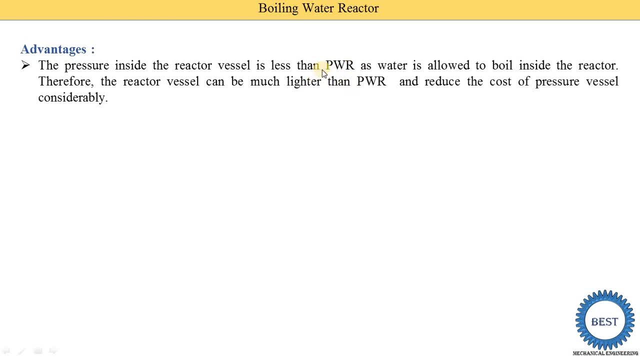 pressurized water reactor means with respect to the pwr pressure. in a bwr means boiling water reactors are less due to these less pressures. the water is boiled inside the reactor. so we know that when the pressure is increased then boiling point of the water is increased. okay, so in a bwr the 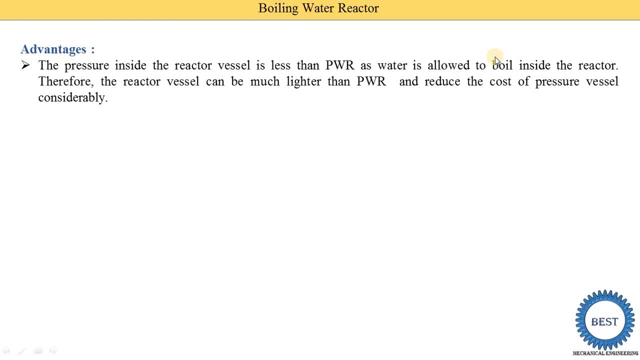 pressure is lower. so water is boiled means water is converted into the steam in this reactor. therefore the reactor vessel can be much lighter than the pwr and reduce the cost of the pressure washer considerably means when this pressure is high we need to use the larger thickness of the tube or we are required. 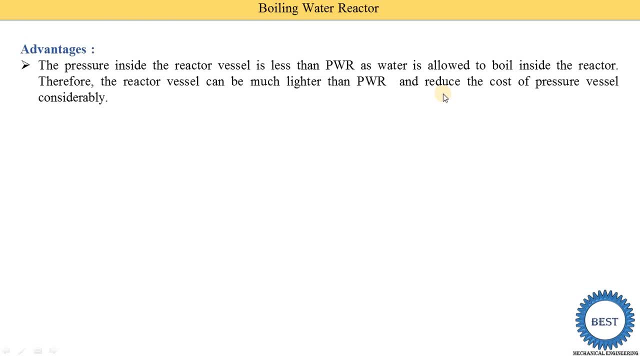 the larger thickness of the shieldings. so in a bwr the pressure is lower, so cost of the construction is reduced. it eliminate the use of heat exchanger, pressurizer, circulating pump and the piping. therefore the cost is further reduced. okay, so here you see. this is the diagram of the pwr. so in a pwr, here you see this. 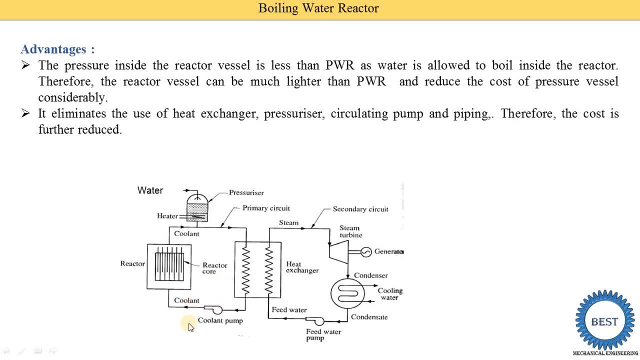 pressurizer is there, this heat exchanger is there, circulating pump is there means coolant pump is there, okay, and the piping is also there. so these things are increase the cost. but in a bwr only reactor is there then steam turbine, condensers and piping is also there. so these things are increased. 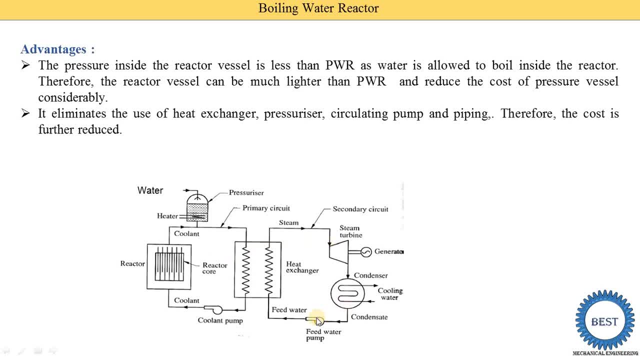 the cost. but in a bwr only reactor is there, then steam turbine condensers and circuits are also there, then steam turbine condensers and the feed water pump is there. so cost is reduced compared to the pwr. the thermal efficiency of this reactor plant is considerably higher than the pwr, so in 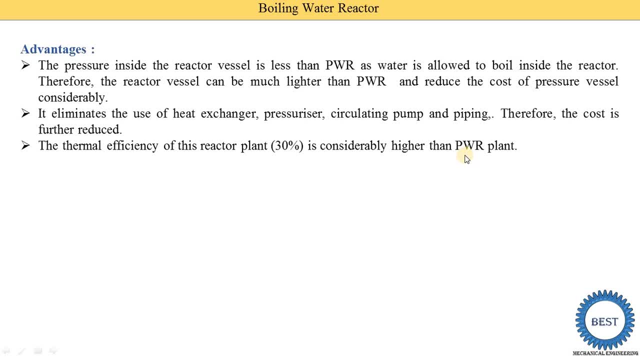 a pwr efficiency is 20 percent. okay, here the efficiency is 30 percent. means efficiency is improved by 10 percent. the temperature remains low for the given output conditions. next one is the disadvantages. first disadvantage: the steam leaving the reactor is slightly radioactive. therefore light shielding of turbine and the piping is necessary. means 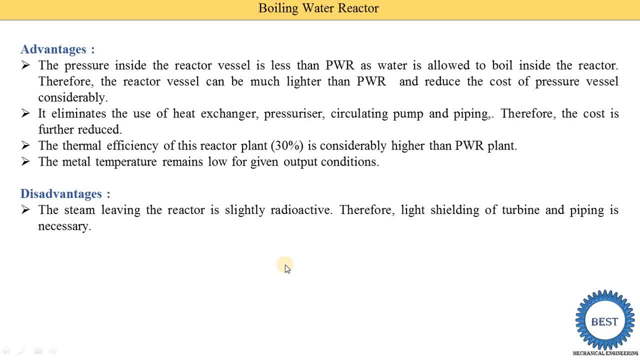 we need to shielding the full plant okay. so in a pwr, just we need to shielding the primary circuits, okay, but in a pwr we need to cover the full plant by the shielding. full plant means we need to cover all the components by the shielding, that is, a reactors, turbine, condensers. 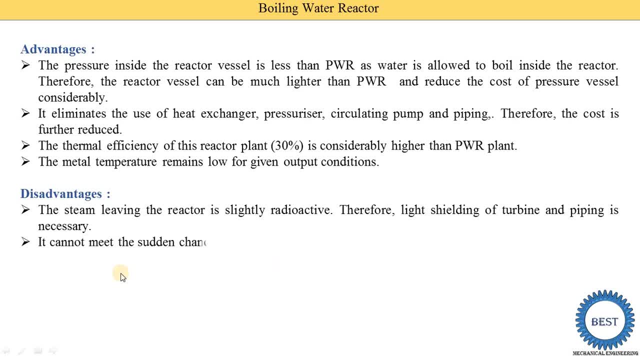 and the pump it cannot meet. the sudden changes in a load on the plant means if the load is changed, means electric load is increased or decreased. so plant are not able to give the quick response. the power density of this reactor is nearly 50 percent of pwr. therefore the size. 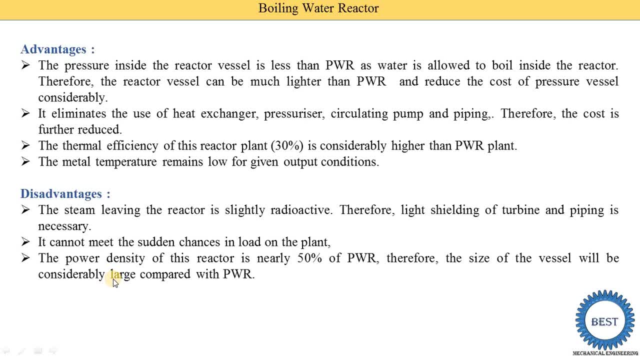 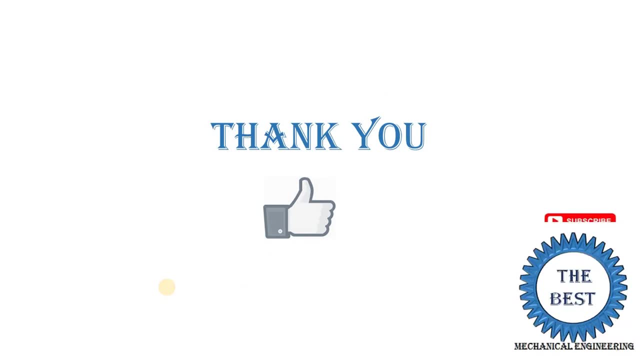 of the vessel will be considerably larger compared with the pwr. its require energy of the pwr and in this pwr we are not able to use the natural uranium. we are using the enriched uranium as a fuel. so thank you for watching this video. if you learn something, 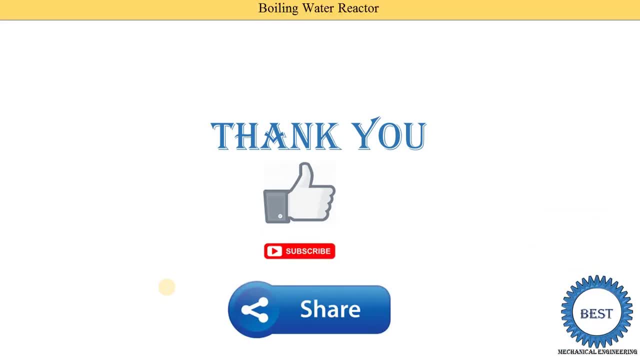 then like the video and share the channel with your friends.